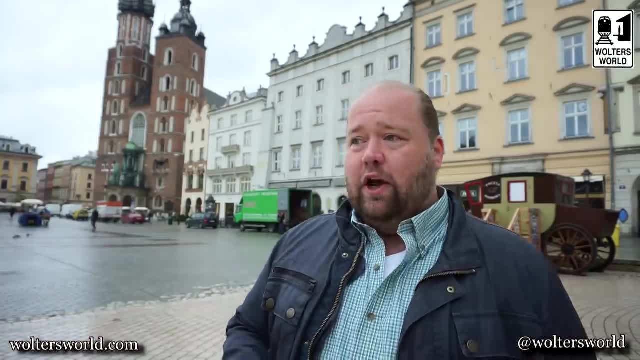 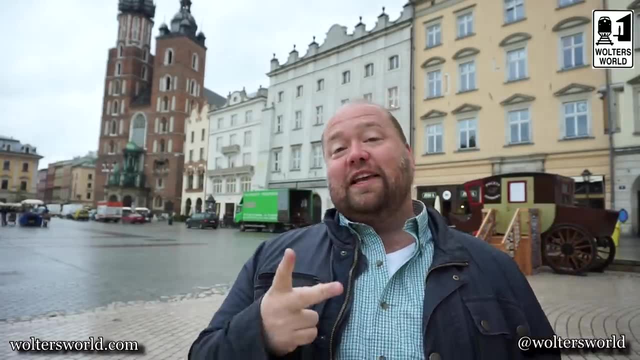 also kind of shocks the people when they come here, because I'm used to all those Polish jokes where- what is it? four Polish people and how do they, you know, move the bed or something? You don't have that here. The second thing that'll shock you when you come here also deals with the Polish people, are how 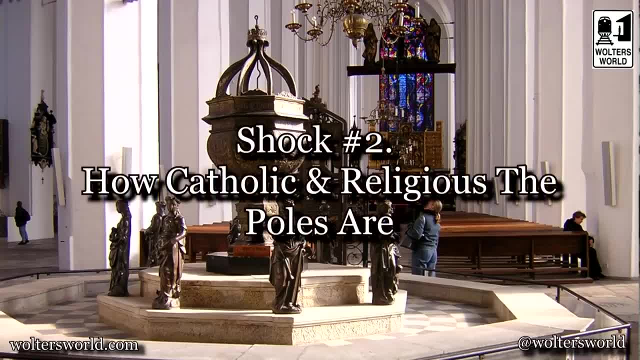 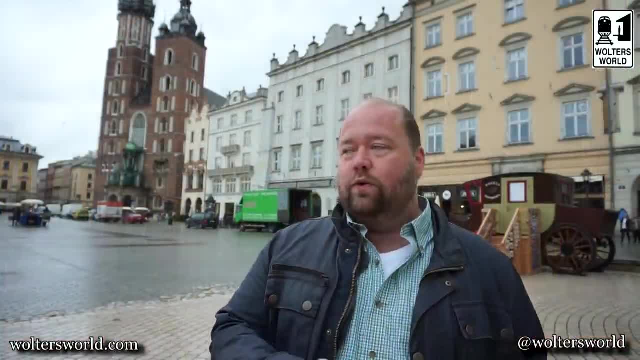 Catholic and how religious the people are. I mean, I remember going on the buses in Lublin and these like punk rock guys are on the in there and and they go by a church and they all do the sign of the cross. I'm like whoa, I didn't expect that. People here in Poland are very religious And 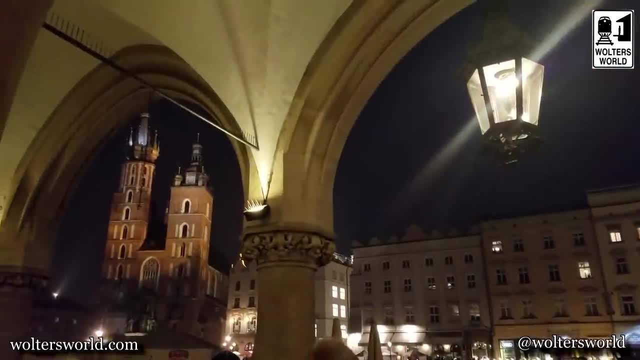 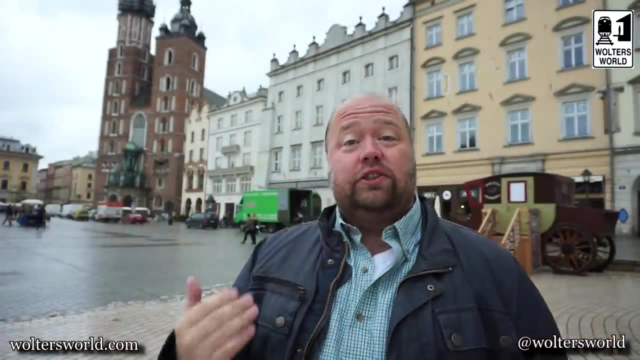 the churches. this is St Mary's. Honestly, the first time I walked in there 20 years ago, I would just draw a drop: Wow, The blue, the all blue altar and the blue ceiling and everything. And the churches around the country are gorgeous And they're actually building more churches here. 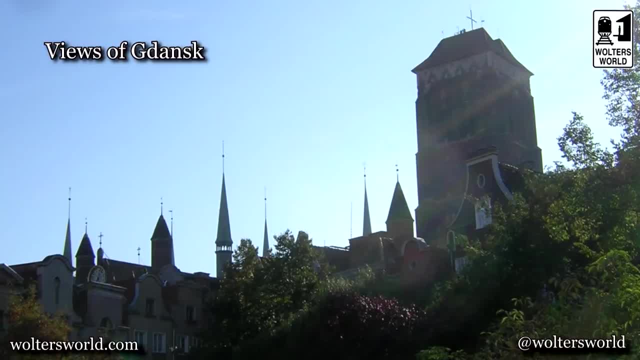 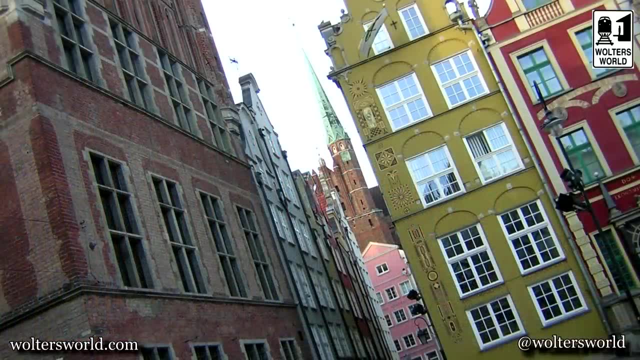 You know other countries. they're turning churches into apartments and hotels and bars. Here people still go to church, They still do believe And you do have a very religious conservative feel. when the people are here, which is kind of a different thing, And you go, and when 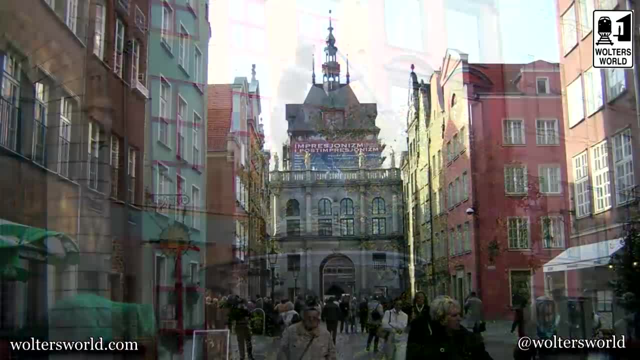 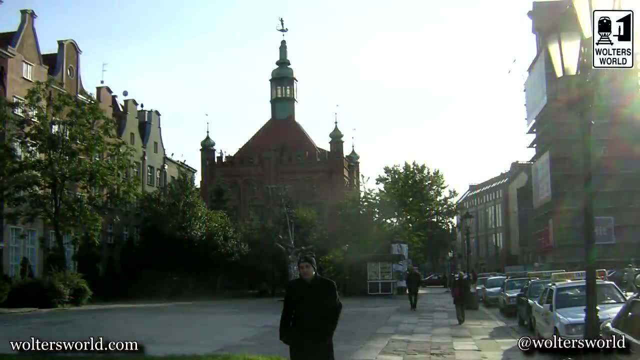 you go in the churches. that's the real thing about it. You really see the beauty of the churches, The ones that haven't been destroyed during the war, um that may, they've been rebuilt, but like here and other ones, you really go in and just see the. 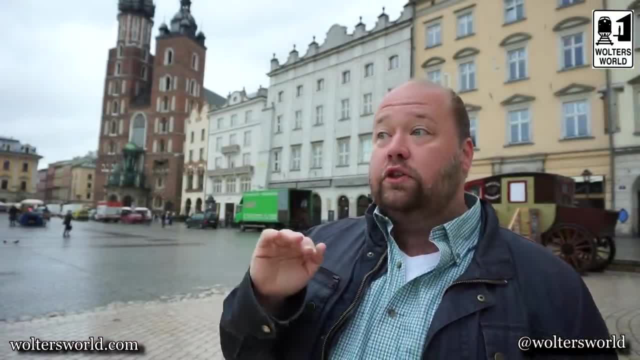 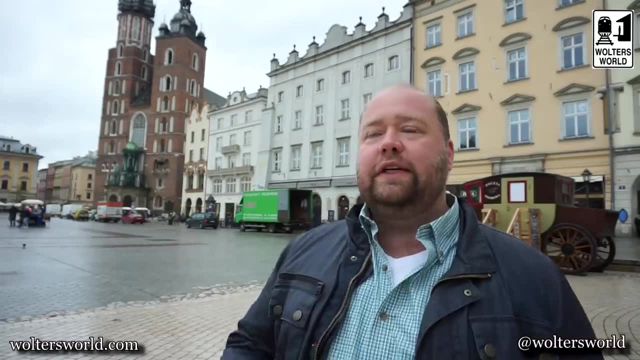 The majestic beauty of the churches here. So do take the chance to go into the churches, Don't just go. oh it's another church, Go in and check it out. And that kind of leads into the third thing that'll shock you when you come to Poland is how much Poland was destroyed during the Second World. 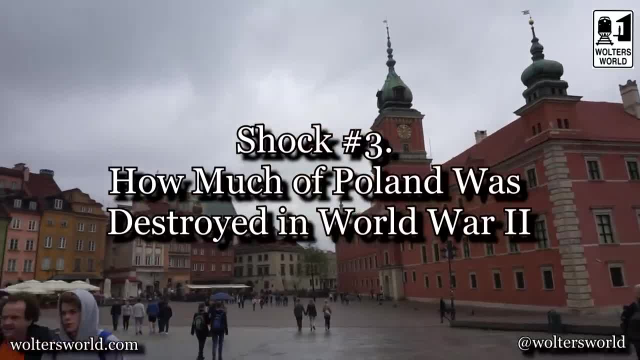 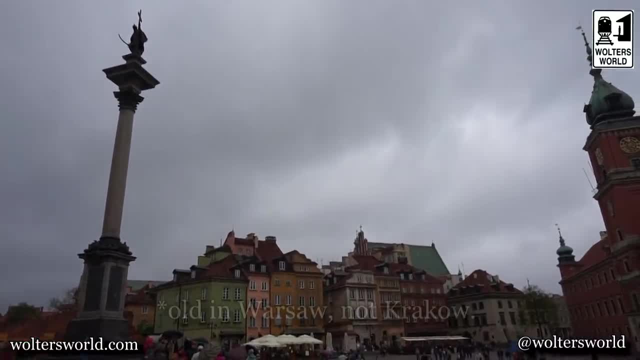 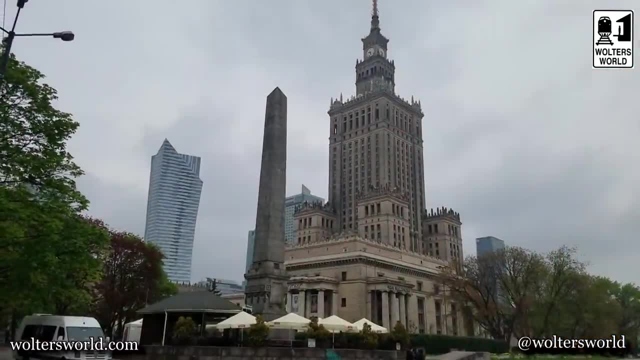 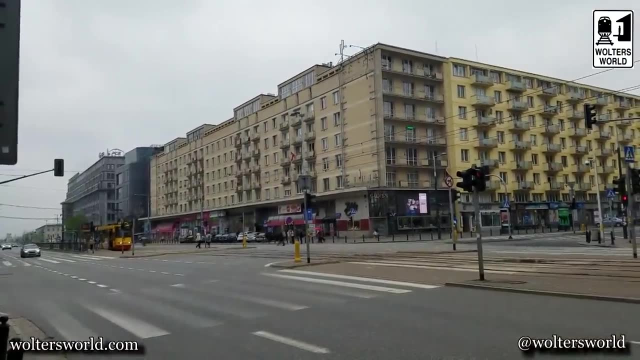 because it got leveled by the Nazis, And you'll see that and you go around. that's why you'll see that communist architecture in the big square, long rectangle buildings and stuff like that, Because there was nothing there, It was all. 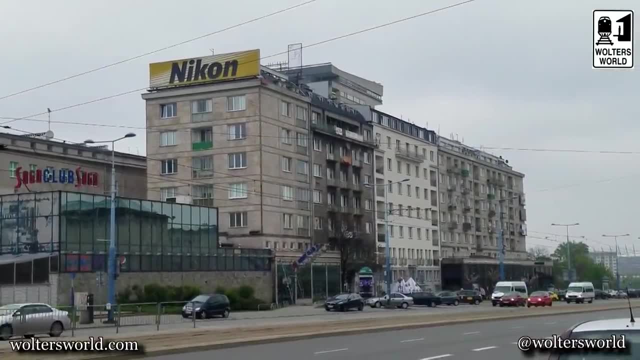 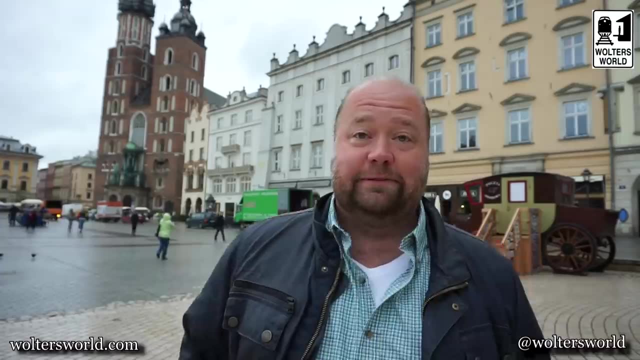 destroyed So they had to rebuild. And when you really see the level of destruction throughout the country and how much they've come back and built new stuff, you'll be very proud of the people, and that's what's really cool about it. Now the fourth thing: that's going to shock you. 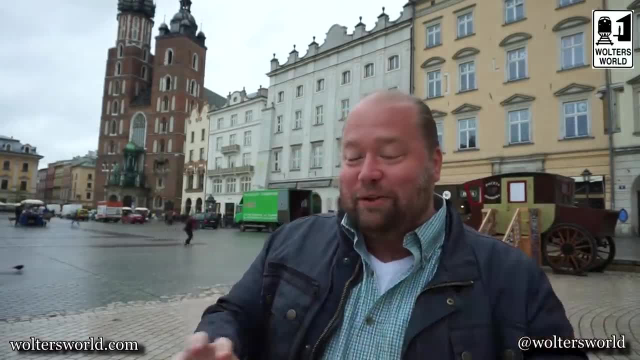 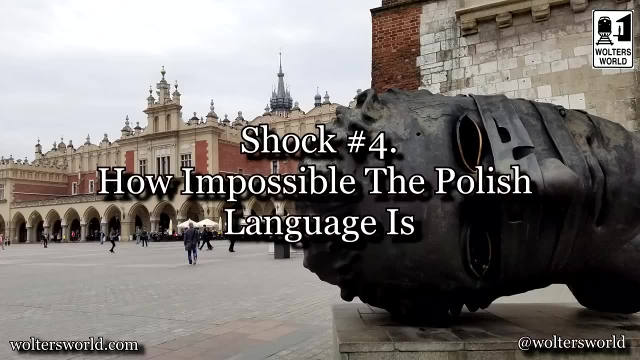 when you come to Poland is how completely incomprehensible and illegible the Polish language is. Look, if you don't speak Polish, it's okay, The locals know you don't speak Polish. They'll still try to speak Polish with you, But Polish is just one of those. 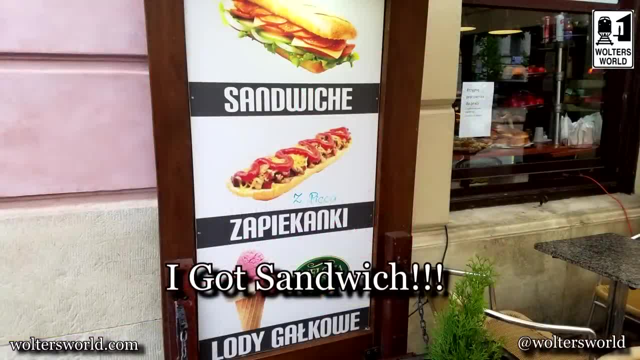 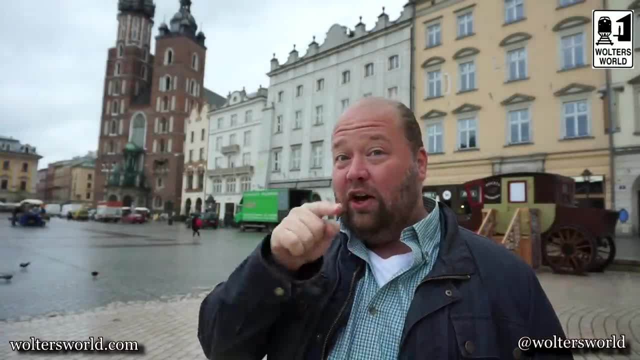 languages. you're listening at the train station you're like, yeah, I got nothing. Yeah, I got. I don't even know what city I'm going to. It is a very tough language and it's very hard to pronounce. Like how do you say P-R-Z in a row? And there's like 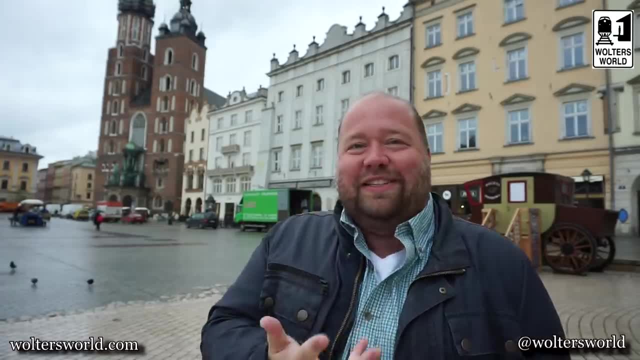 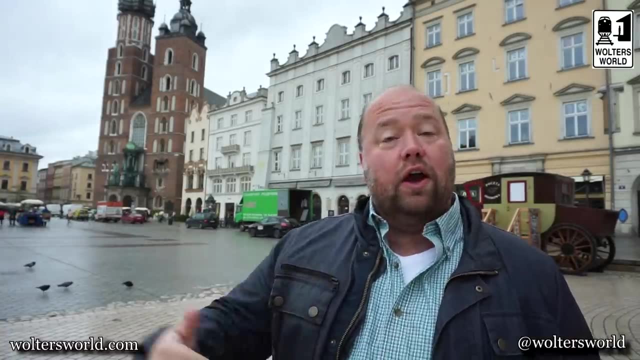 a hat and there's an L with a line through it. Is that a T or a W? What is that? You do get pretty confused when you are here and it is kind of shocking that you can't even make out some of the stuff. Now they are developing better for tourism. 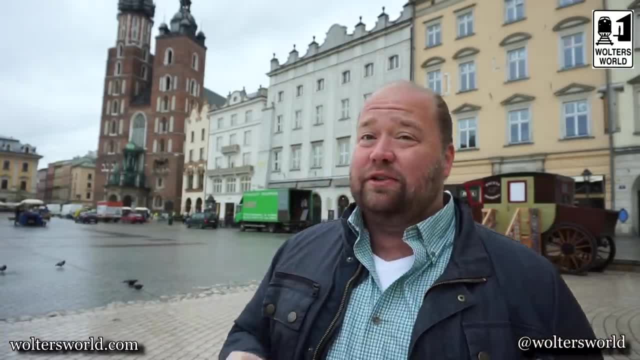 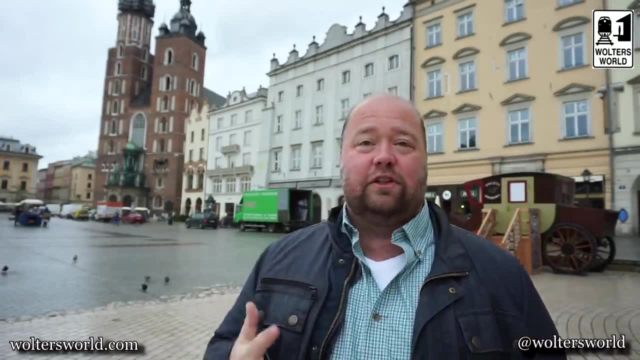 so you will have a lot of you know English menus and stuff like that, But it is a really good idea to know some Polish before you come. like dziękuję, which is like thank you, prosim, is please, things like that, because it really gets. 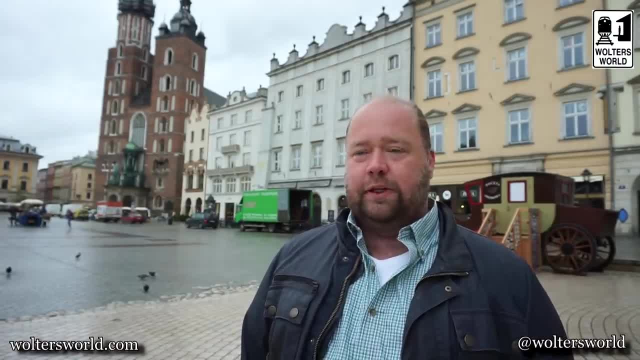 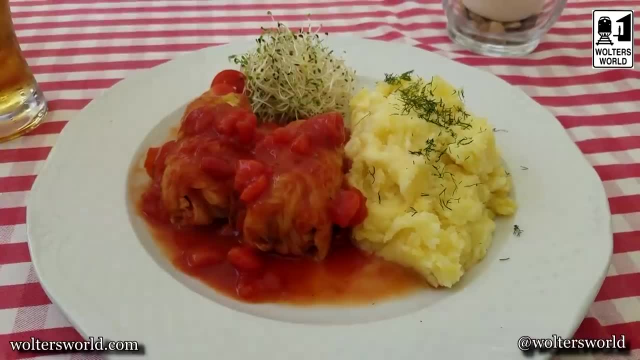 those people to go from you say: dwa piwo prosim. Oh, you speak Polish And they really open up. then okay. The fifth thing that might shock you is your eating experience here. The Poles really love their potatoes. They love their potatoes. 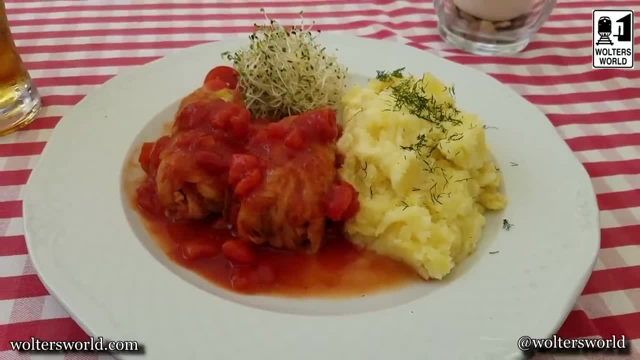 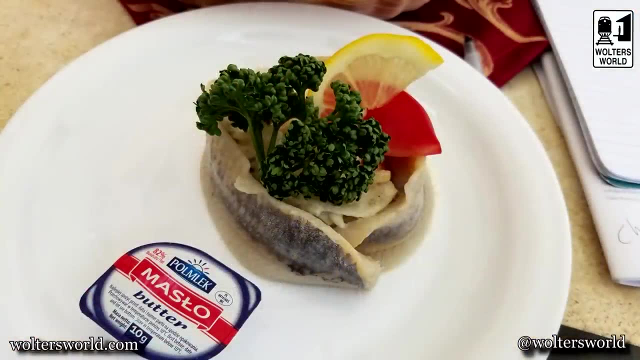 And their cabbage. And even if it's not on the menu, like it may say: oh, it's a cutlet Nice, It'll come with cabbage and potatoes. You're like, oh, I'll have the pork knuckle instead. 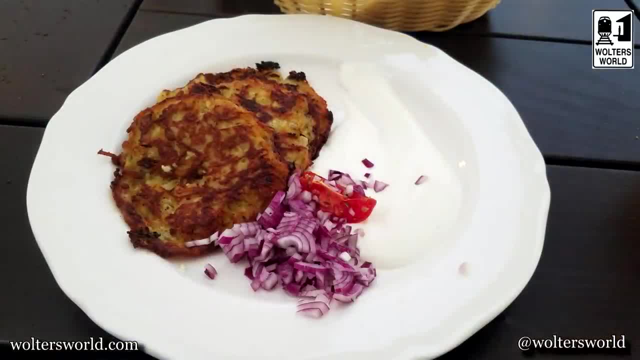 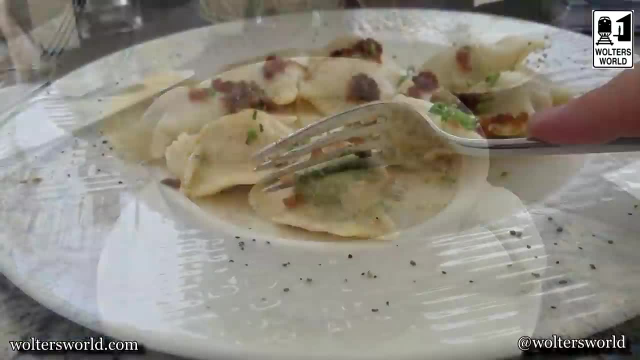 Oh, it comes with pork and cabbage. Well then, I'll just have the rolls. Oh, it's a cabbage roll. Okay, Look, you're going to have a lot of cabbage. You're going to have a lot of potatoes when you are here, And there are some pretty good. 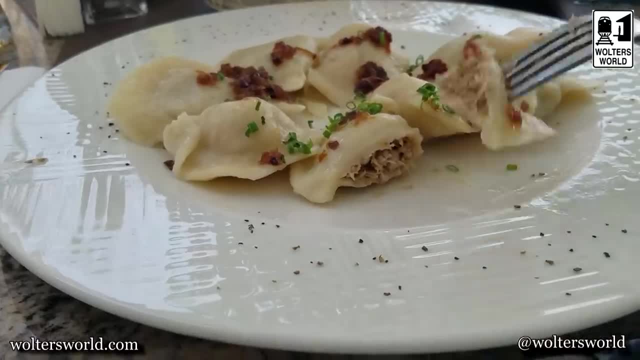 foods like the pierogi. You're going to have that when you're here. I've actually liked the meats when I was here too, And they do a good job with the potatoes, but it's all the time with the- with the cabbage and the potatoes again, and 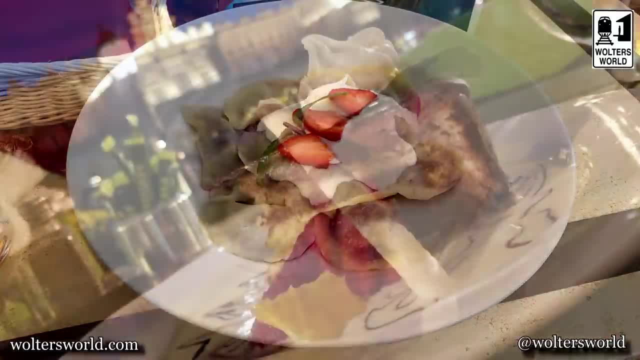 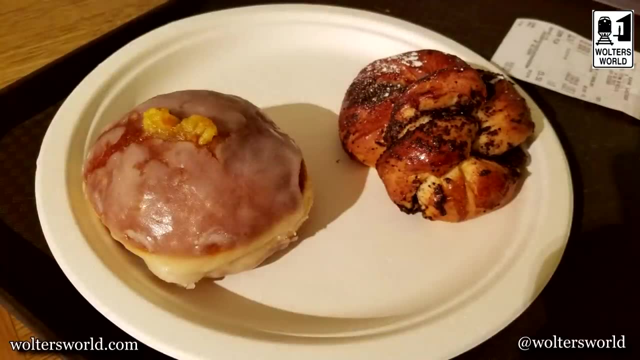 again and again. That's why yesterday I just got the cabbage rolls. I'm like, look, because then I know I'm getting the cabbage, Haha. But it came with a side of mashed potatoes And I just laughed and laughed and laughed- Okay, Also, kind of. 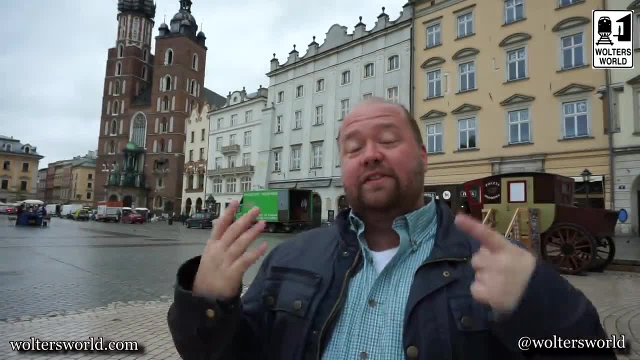 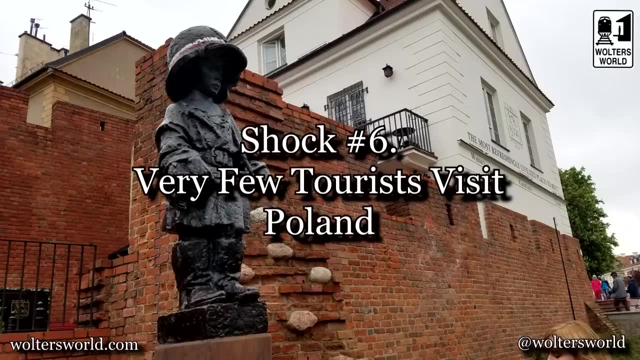 interesting is they really love their tea here too. Now the sixth thing that might shock you as a tourist is: you notice there's not very many tourists Now in Krakow you do get about 10 million tourists a year. I mean, this is a very popular. 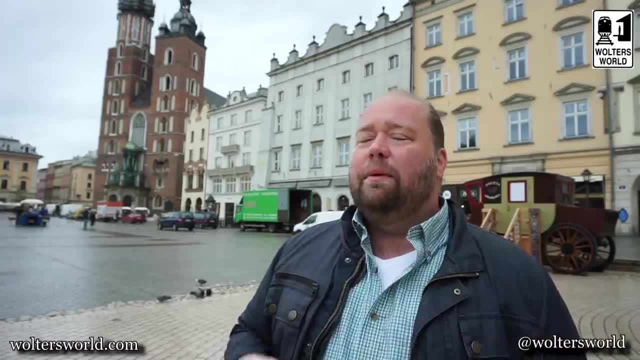 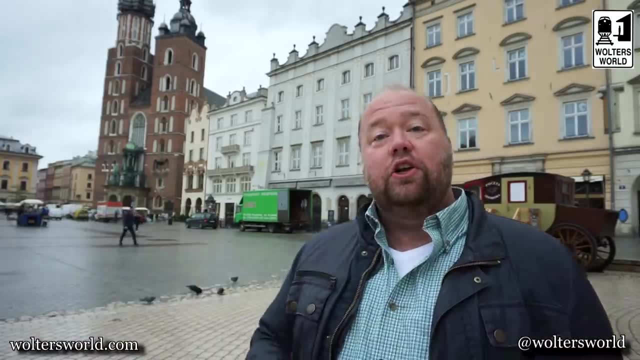 place because it's gorgeous. Think about that towards the end. But honestly, there's not a lot of tourists that actually come to Poland And so when you go around, you really are kind of a special tourist because you're actually here. You might get people going. why are you? 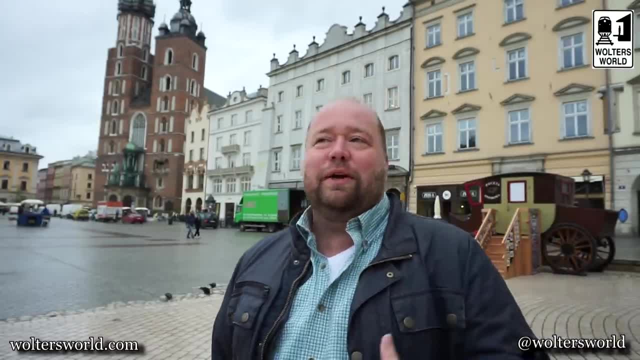 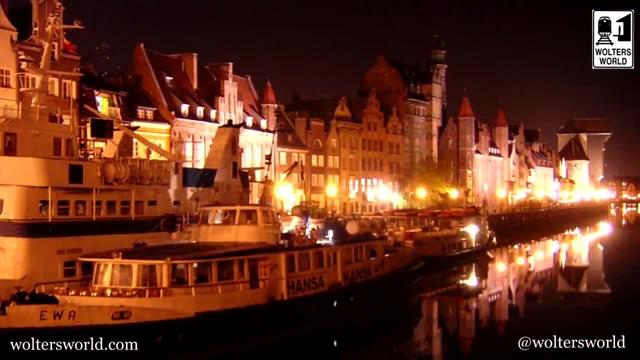 in Lublin? Why- why are you in Łódź? Why are you here? You know some places like Krakow, it's obvious, you know. but you go around and there's just so few tourists out there that you're like, hey, I can kick back, relax and do okay, And 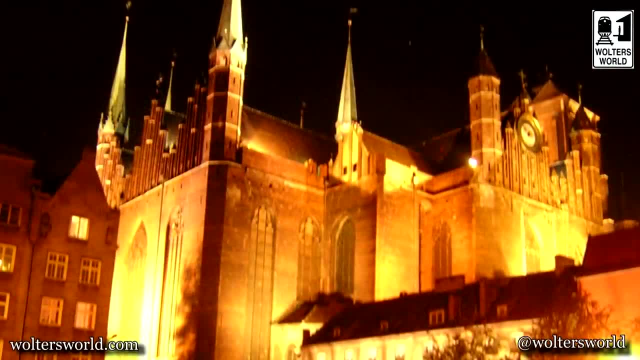 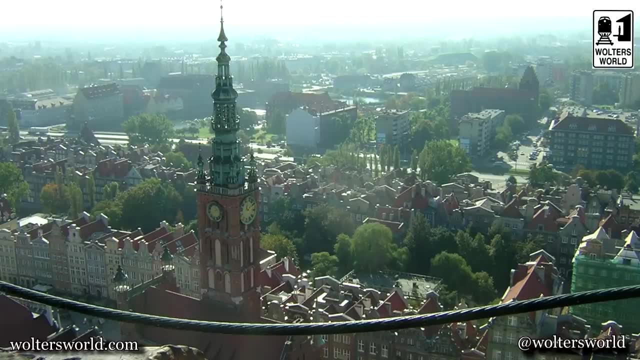 what kind of leads on to that is. our next shock is how cheap it is here, Because there's not a lot of tourists driving up the prices. It's nice because you can have a very affordable vacation here in Poland: Rooms, accommodation, food, drink, making, merry all. 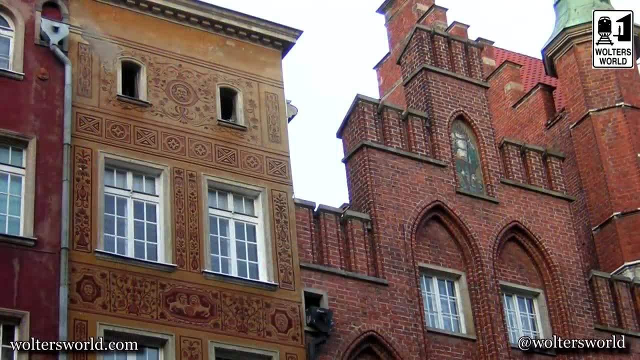 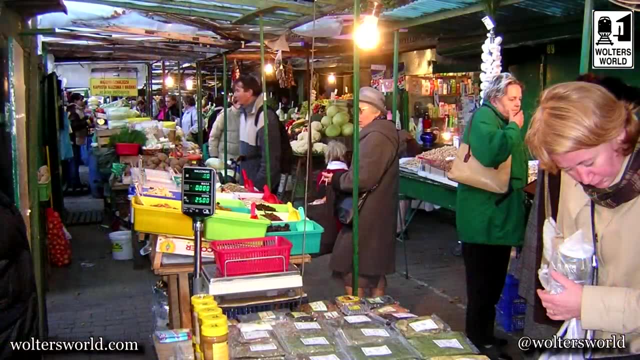 kinds of stuff And you'll see a lot of people come to like Krakow or Warsaw to come have a party weekend and stuff like that, because you really can. Your money goes a lot farther here than other places And that's what's really cool Now. 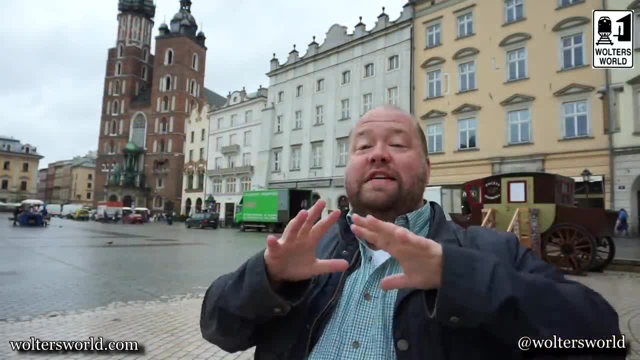 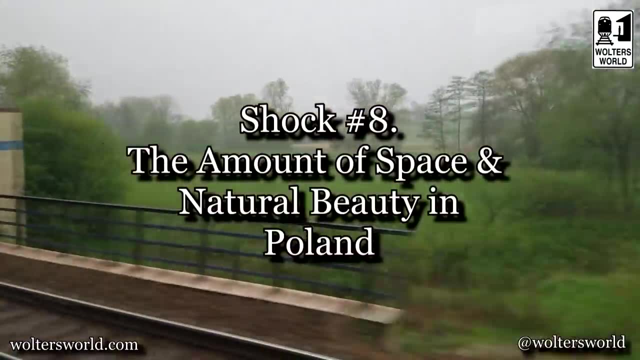 the next thing that's going to shock you when you are here is the amount of natural beauty and space in Poland. Look, this is a huge country. It's one of the biggest countries in Europe, And the thing is you're going to be going between these different towns. 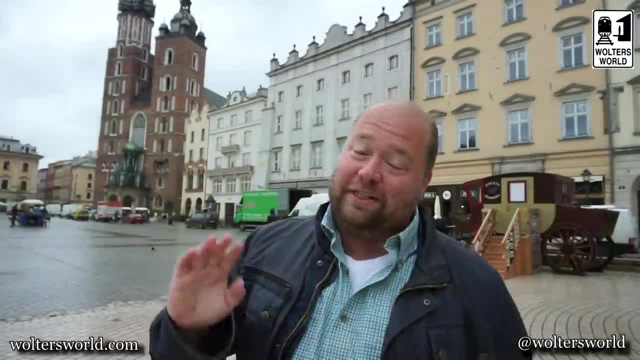 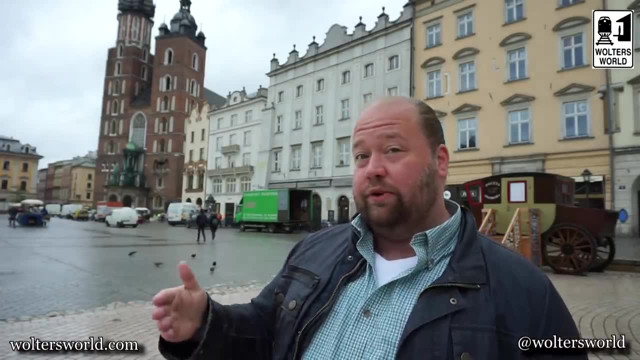 whether it's on a bus or a train, things like that- Not super fast trains, but fast enough trains And you're going around and it's just amazing how big the country is, but also the natural beauty you see when you go through there And what's. 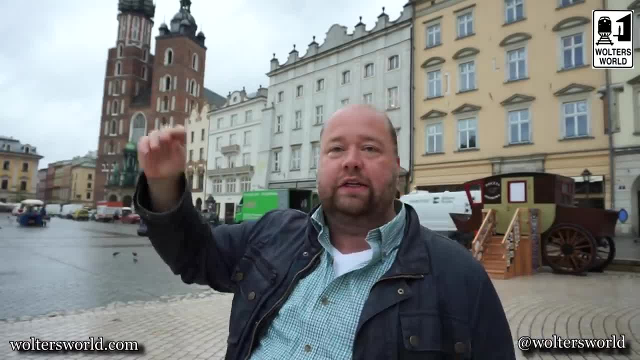 nice is when you go through and you can go. if you're in the Indian North, you're going to Gdansk. That's one of my favorite. Krakow and Gdansk are my two favorites. You're up in Gdansk, you come down a bit. you can go over the Missourian. 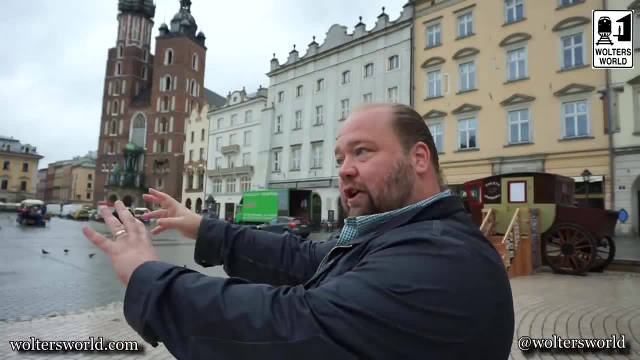 Lakes and see the, the castle that's right by there, the Marlborough Castle, which is on the way towards there. Go to the lakes and enjoy that. Go to the coast in the north, In the south you've got the Tatras Mountains. You go to Zakopane to. 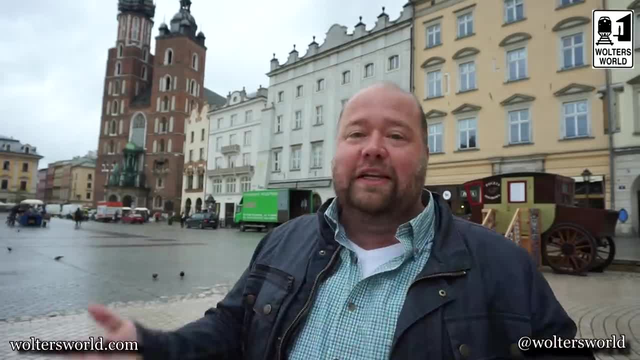 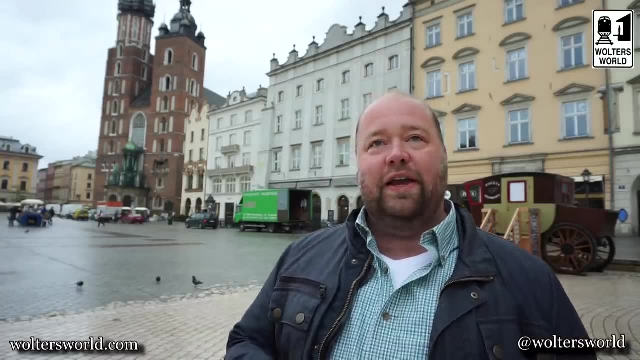 stay there. Tons of Europeans go there to ski in the winter because, yes, it's beautiful and it's cheap. Remember what I said before. But you have this natural beauty like wow, this really is. I understand why they have all their tourism propaganda. 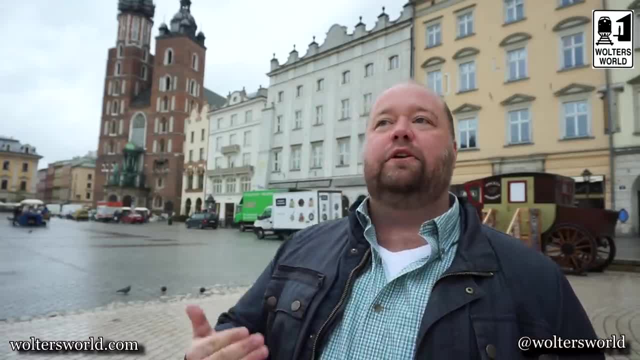 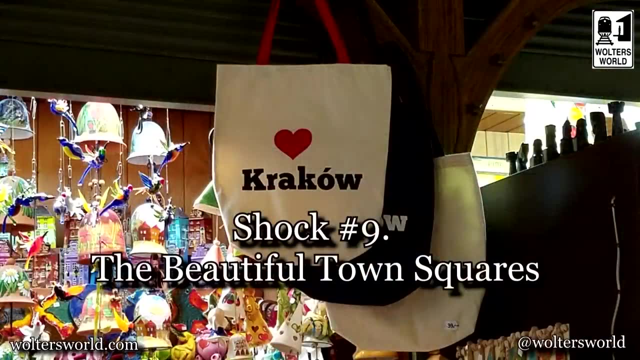 is about you know the natural beauty of Poland, because it really is beautiful. Having said that, the next thing that'll shock you is how amazing the town squares are here in Poland. Yes, here in Krakow, You've got the, the cloth hall, over here to check out. You've got the St. 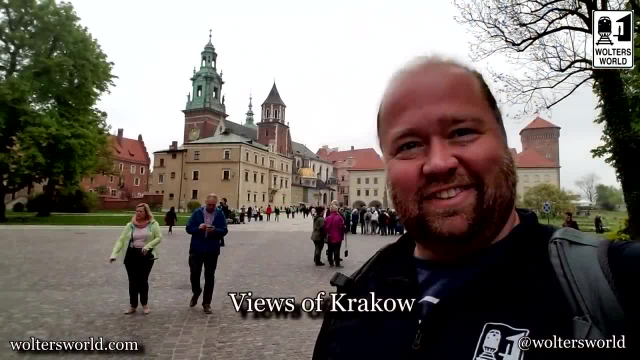 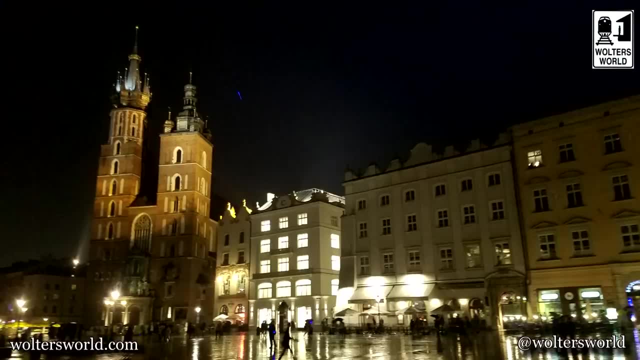 Mary's Church over there. You've got all these things, Sorry, You've got all these things to go and see, And this is actually the largest town square in the European in Europe, And it's amazing, but it's not just here. You go to Warsaw to see their. 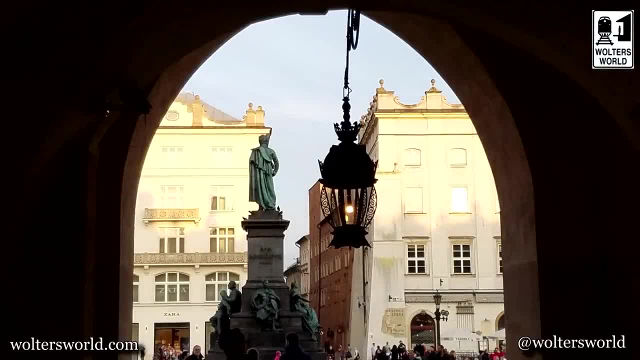 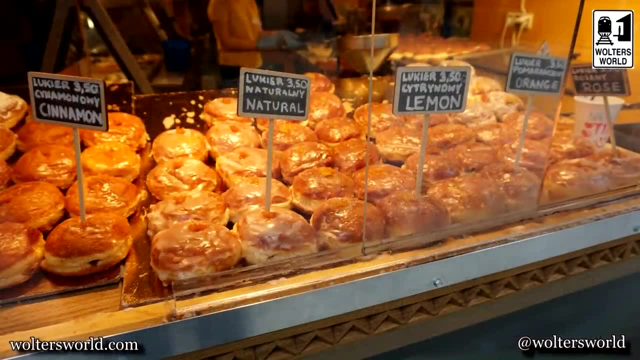 old town square. they really built from scratch. Wroclaw. Go see the old town in Lublin. Oh man, Gdansk, the port city of Gdansk. man, you just walk around there see the Neptune statue. You're like man, this is so cool And you have. 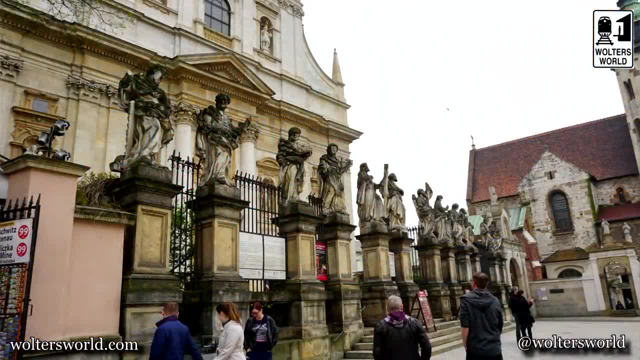 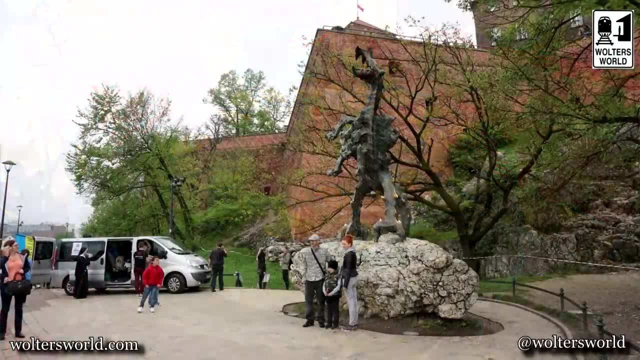 all these beautiful squares and you have all these beautiful buildings that have been rebuilt after the war- or maybe they're still there- from before the war. You have that beauty that not a lot of people think of, Because when they think of Poland, you're thinking of you know. oh, it's just, it's farmland and 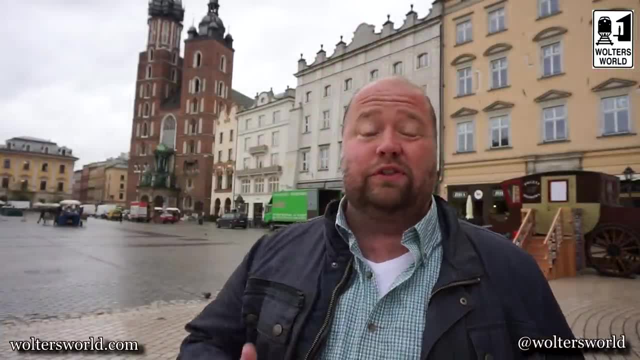 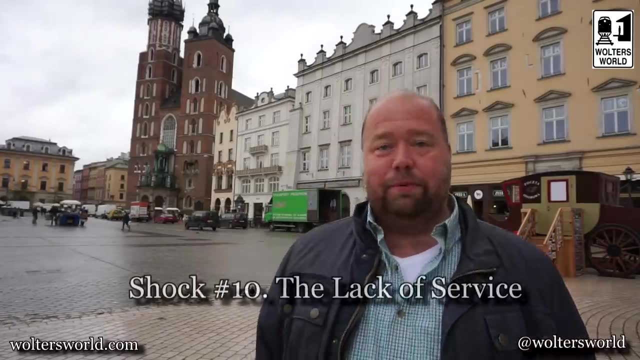 stuff like that. And look, there are some just amazing places here in Poland, So it's definitely worth checking out. And the tenth thing that might shock you when you do come to Poland is the lack of service. So remember that Polish face. 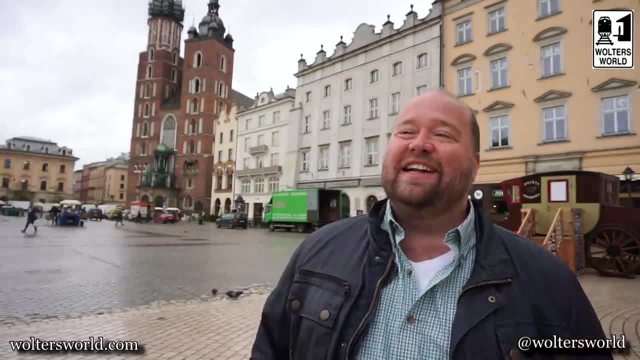 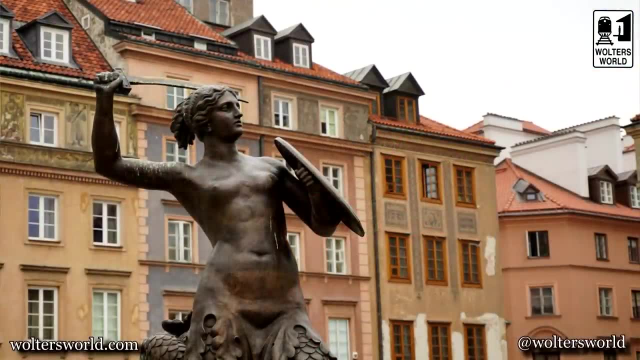 This is your service. It's not the most attentive, It's not the most friendly. You'll get your food, It'll just take some time. But just know Poland isn't necessarily the most service oriented economy out there, So you need to have some patience when you are when. 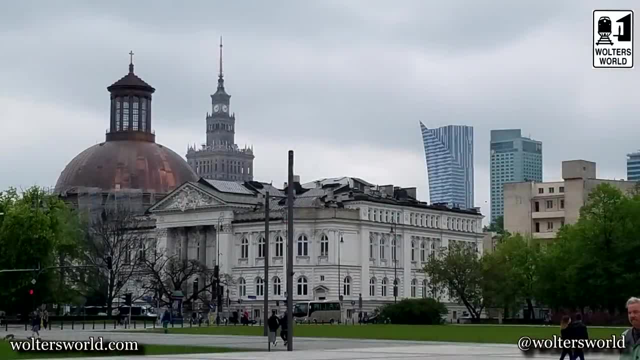 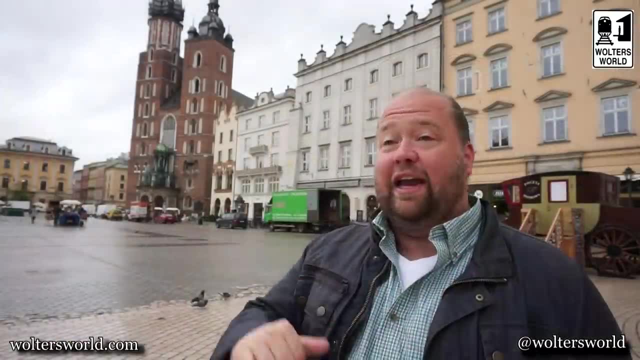 you are coming here And probably that's the only thing that shocks you kind of in a bad way is really the service here isn't the best, but it's getting better. I used to come here a lot in the early 2000s for work And compared to, you know, 2017. 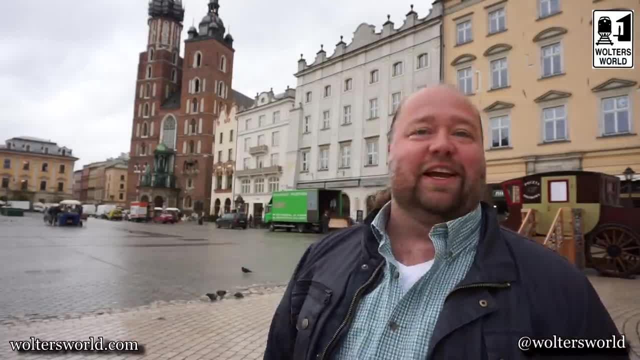 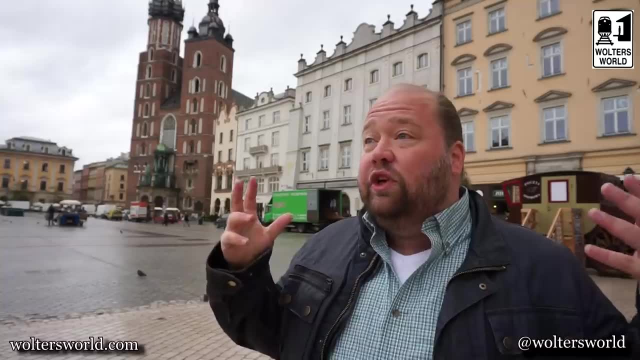 versus 2007 or 2002.. Man, it is, it's completely different. Anyway, I hope that helped you know a few things that might shock you before you come to Poland. It is a great country to visit because you're one of the few tourists coming here to see some of these. 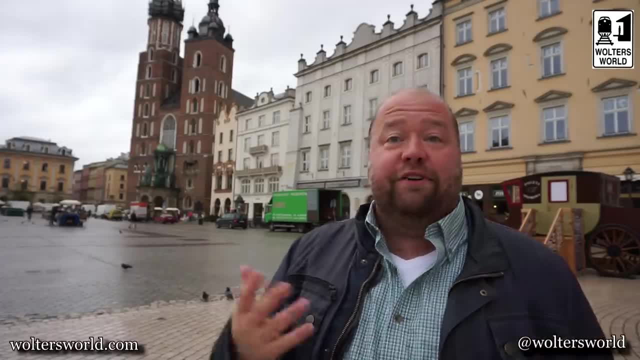 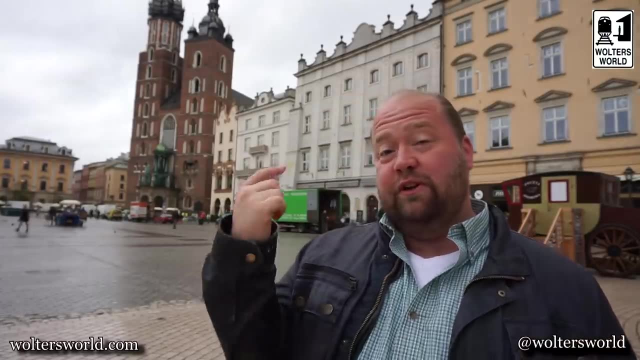 beautiful cities like Krakow. So if you want to learn more five things you love and hate about Warsaw, what you should eat when you come here to Poland, check us out on our website at waltersworldcom. We're also on Twitter, Facebook, Instagram. 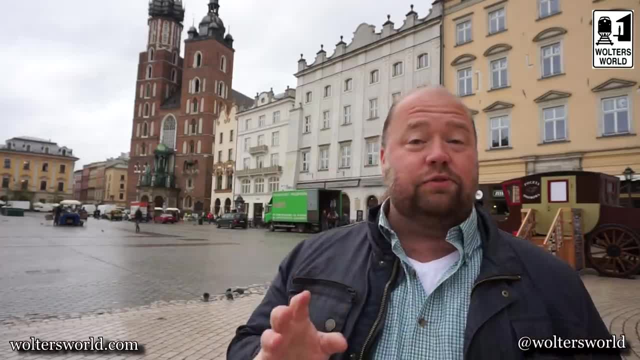 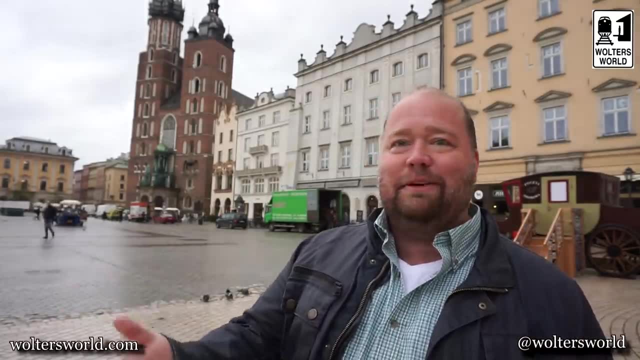 YouTube And we really appreciate your likes, subscriptions And if you do subscribe to our channel. we actually put out two travel videos every week, every Wednesday and Saturday, And we really appreciate those likes. And if you got comments about things that shocked you about Poland, put in that.